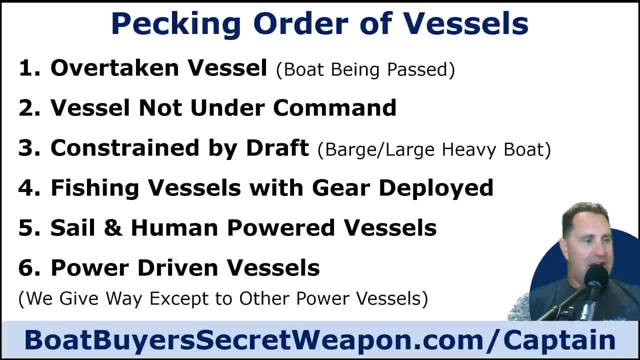 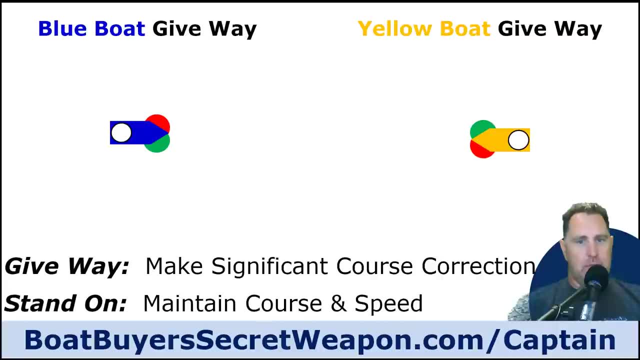 That's all of us pleasure boaters, including personal watercraft. We give way to everybody. We're the give-way vessel to every other vessel in the pecking order. So here let's look at an example: Meeting head-on. When you're meeting another boat head-on. 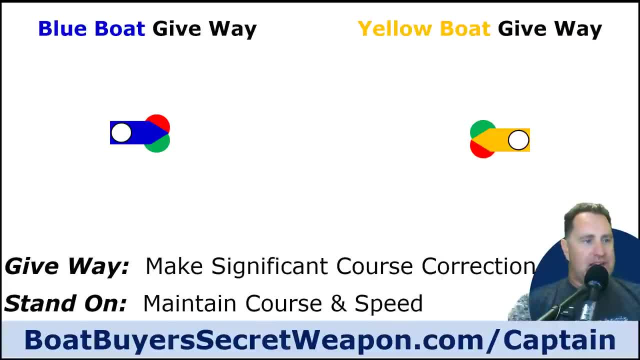 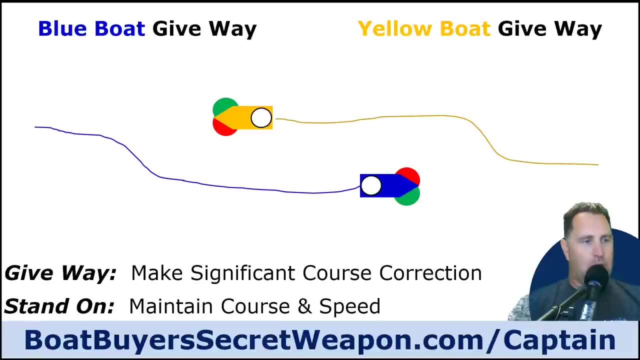 you're both give-way vessels, You both need to make a significant course change to avoid collision and you both go to starboard. You pass port-to-port, you go to starboard and you pass safely. But you can see, it's a significant change in course and then you pass. 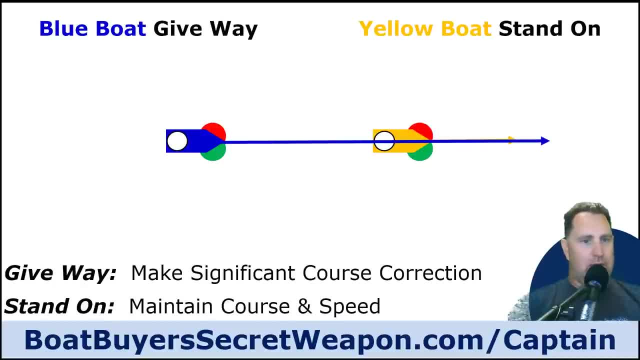 If you are going faster than somebody that you're following. first of all, I recommend don't follow somebody too close, Don't get right between their wakes and get right up on them. That's not a good situation, But you're the give-way vessel if 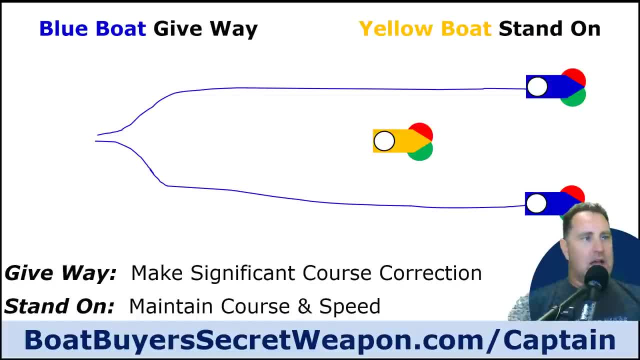 you're traveling faster And what you need to do is again make a significant change. well, behind them, not right behind them, and you can pass them: port or starboard. I am going to recommend that you pass to the starboard if it's safe, if it's possible, because that's going to give you. 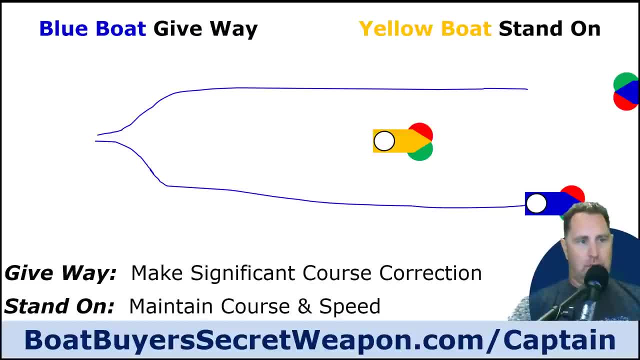 a clear path. And if you do meet another boat, well, you're going to go to starboard Again and you're not cutting in front. If you go port and another boat's coming head-on, well, you're going to have to cut back starboard and you have to cut right in front of. 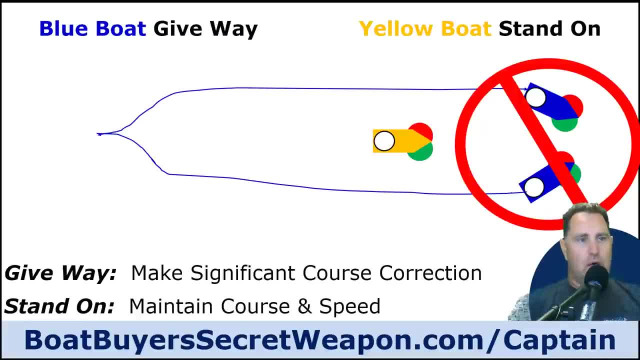 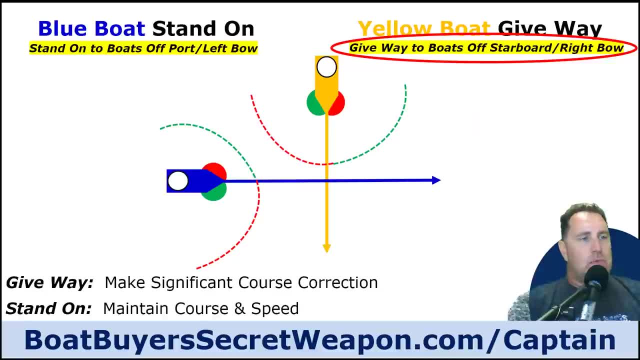 the boat you just passed. You don't want to do that. You want to get well ahead of them before you get back into their line and your wake disturbs them. This is what I think is the most confusing for people is when there's a crossing situation, When you're going. 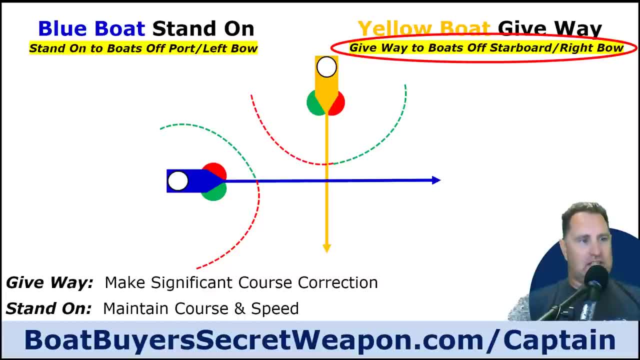 and it appears that you're going the right speed, the right direction, where you're going to cross each other's paths. You're going to go to the right speed, the right direction and you're going to have a collision or near collision. The way I like to look at it is, if you know one, 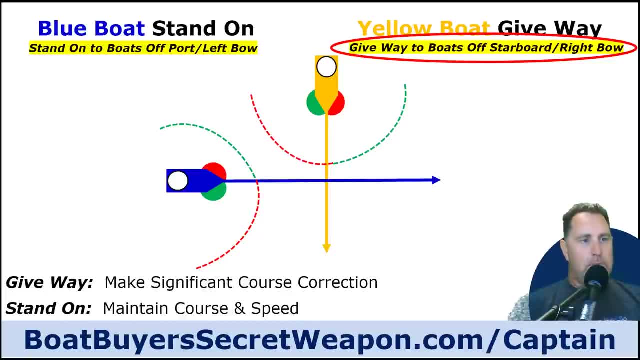 then you can figure out all the rest. If you give way to boats off your starboard or your right bow, so that red line there, if you give way to anybody that's approaching you in this arc, right there, you're going to be the give way vessel and you're going to make a 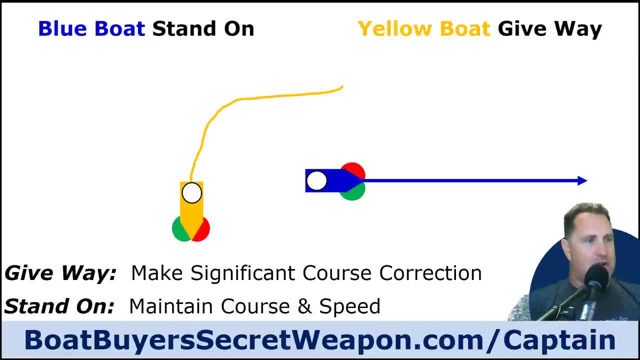 maneuver to avoid them, and it's going to look like this: You're going to make a significant maneuver- starboard- and you're going to pass them on their stern so they can get to the boat. You're going to continue going forward at their course and their speed and you pass them. 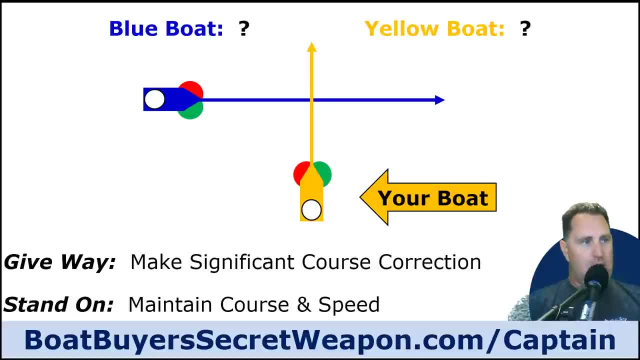 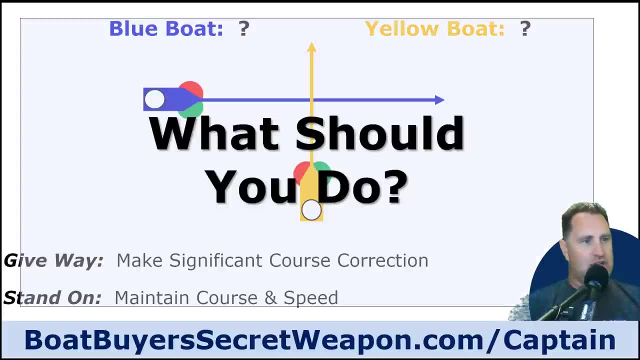 safely. Let's take a look at this example. You're the yellow boat and you are meeting the blue boat. It looks like you're going about the same speed. that's going to make you cross and have a potential collision. What should you do? Are you the stand-on, Are you the give way? and what should? 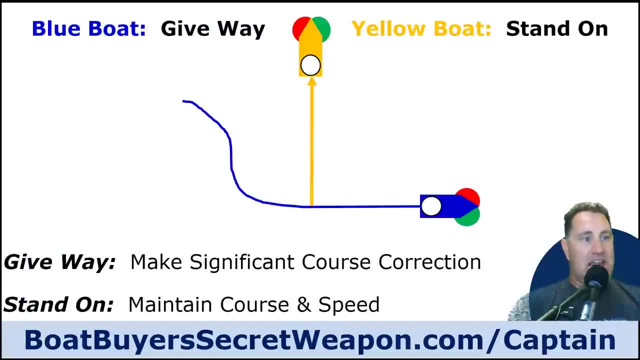 you do. Well, you are, in that case, the stand-on vessel and you need to continue forward. The blue vessel is the give way. They need to make a significant move to the boat. You're going to starboard to let you know. hey, I see you, I'm going this way and pass you safely With the. 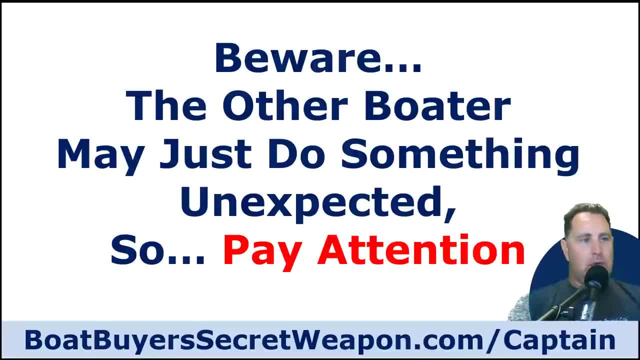 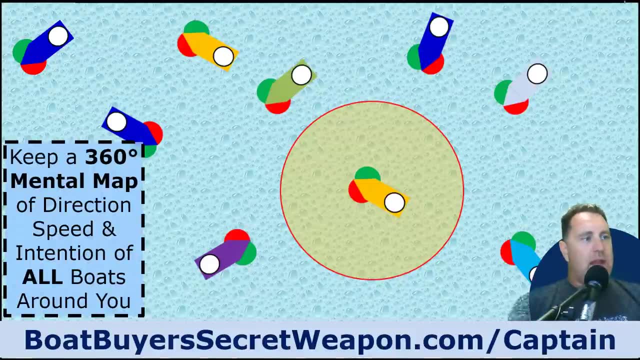 caveat: beware: Some other boaters may just do something unexpected. so pay attention. It's your responsibility to avoid a collision, even if they do the unexpected, the unthinkable, the wrong thing. okay, So here's my recommendation to you. This is what I teach in my Best Boat Captain on. 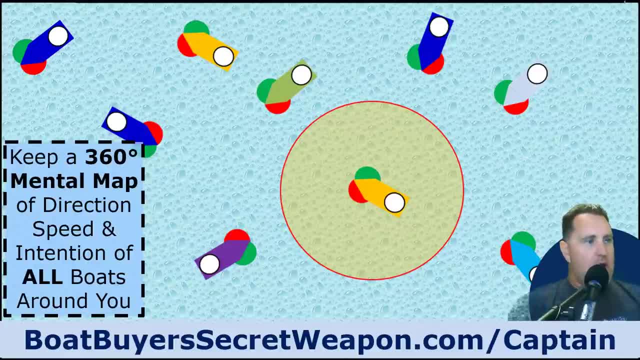 Mental Map of everybody that you can see on the water, their direction, their speed and their intention. What I mean by intention is: what are they doing and what are they likely to do? So if they're doing water sports, what are they likely to do If they're tubing? you know they're. 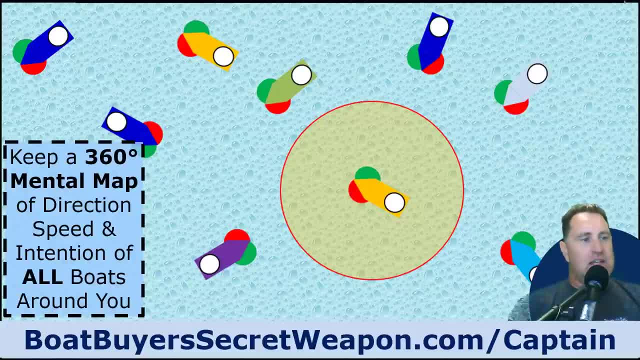 probably going to do some circles and drive radically. If it's a 19-year-old kid in a wake boat or a speed boat, well you know that they might go a little faster. If they're a retired couple in an old pontoon, they're probably going to go slow. So keep that in your head. 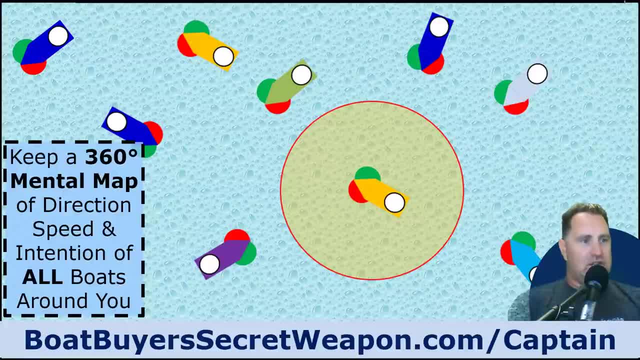 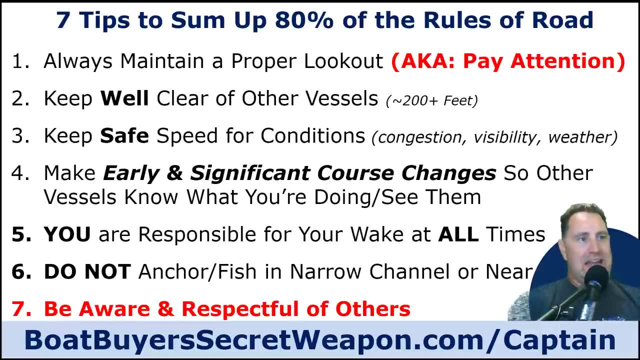 as you're cruising and know where the boaters are, what they're doing, what direction and kind of what to expect from them, and that's going to keep you safe in a lot of situations. So the seven tips to sum up 80% of the rules of the road. Number one: always maintain a proper lookout or pay. 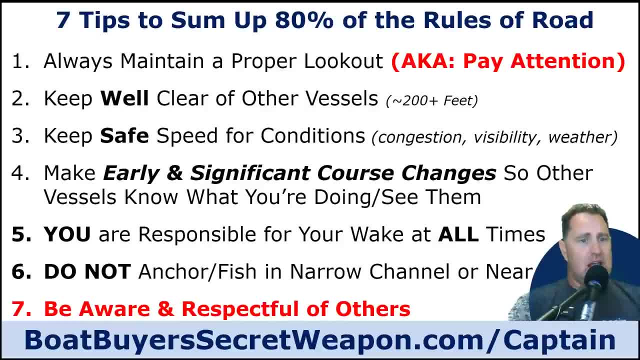 attention. The US Coast Guard releases accident numbers and fatalities and, like the top three, four or five- I've done a video on it- are because the boat operator is not keeping a good lookout or not paying attention. So if you do that number one, you're going to be in great. 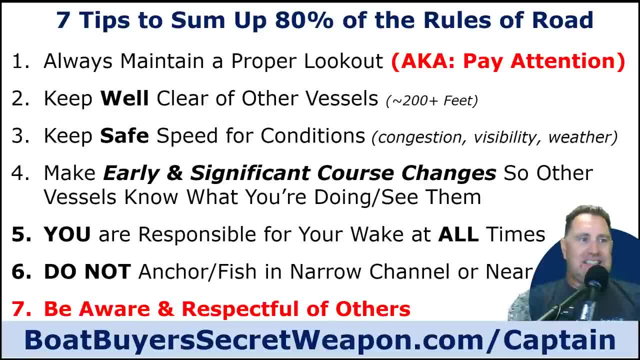 shape. Stay well clear of other vessels. I say 200 feet, No matter what the law is. there's a lot of water out there, Use it and there's no reason to go close by another boat. Keep safe speed for the. 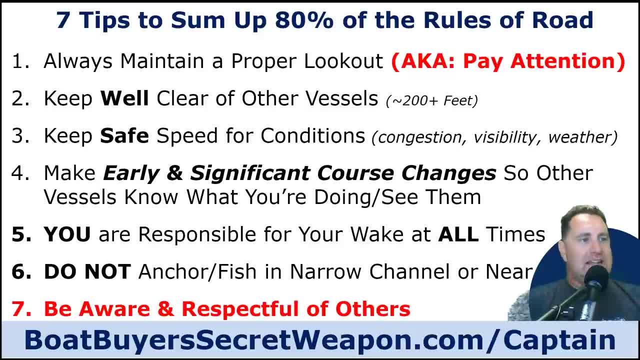 conditions- congestion, visibility, weather- Make early and significant course changes so the other vessel knows what you're doing. You're basically saying, hey, buddy, I see you, I'm going to do this and you do that. It's kind of letting your intentions be known. You're. 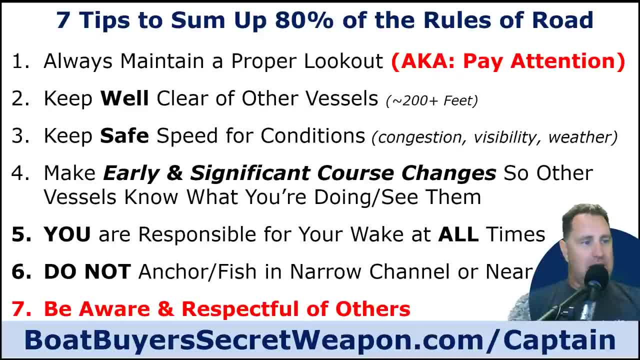 responsible for your wake at all times. whether you're in a surf boat making a huge wake with your ballast, or you're just a boat going too fast but not fast enough and you're plowing the water, Come back on that throttle to get all the way to no wake. and because you're responsible, 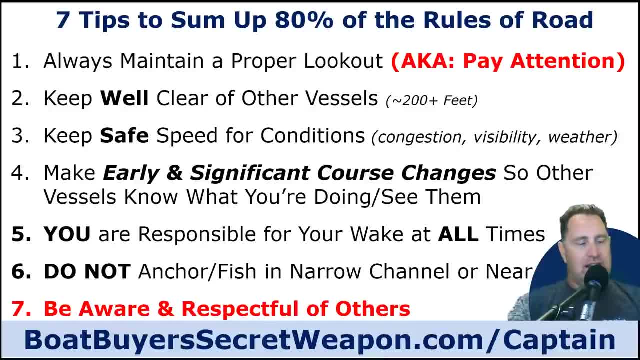 if you're awake at all times, don't anchor our fish in a narrow channel or near a bridge. It's a dangerous area. It's inconsiderate. It's a dangerous area. It's a dangerous area. It's against the regulations. Be aware and be respectful to others. If we all do this, 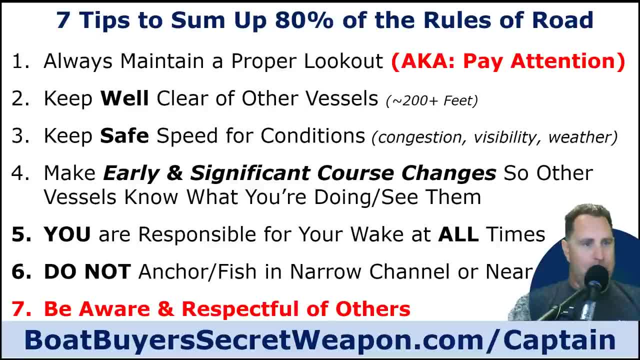 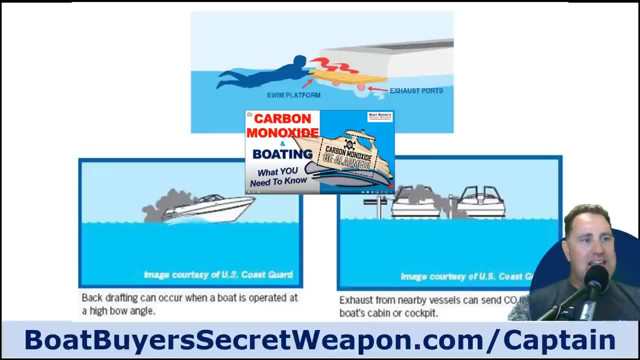 if we're all aware and we're all respectful, everybody's going to have a better time. Now, this is something I created a video on: carbon monoxide and boating. what you need to know, It's the hidden danger of boating. Any motor that runs gasoline creates carbon monoxide. It's 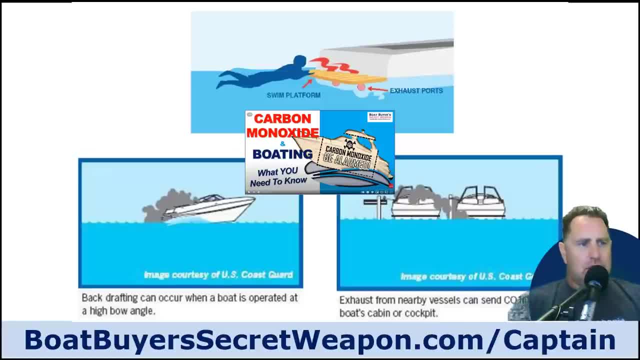 a deadly gas and if you're in a boat- typically a stern drive, on an inboard- you're going with a tailwind, It can blow that carbon monoxide back in the boat. If you're going five, seven miles an hour, wake surfing that kind of speed, it can blow those back in the boat. 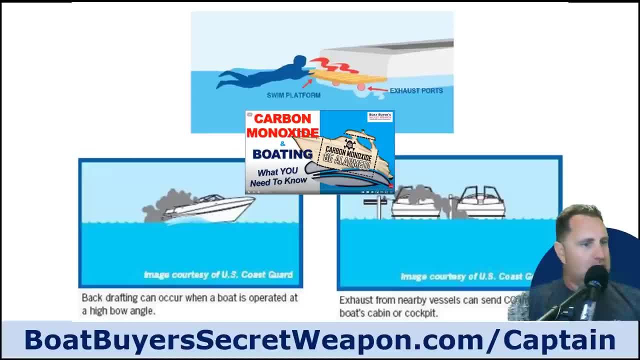 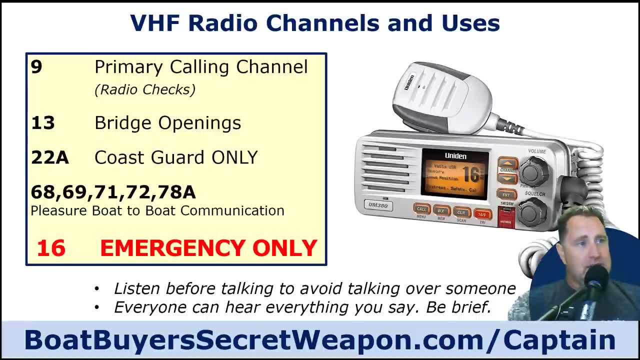 and it can cause major, major problems. Go watch that video. I don't want to go into a lot of detail, but check out that video so you're aware of it. VHF radios: if you need to use it, you need. 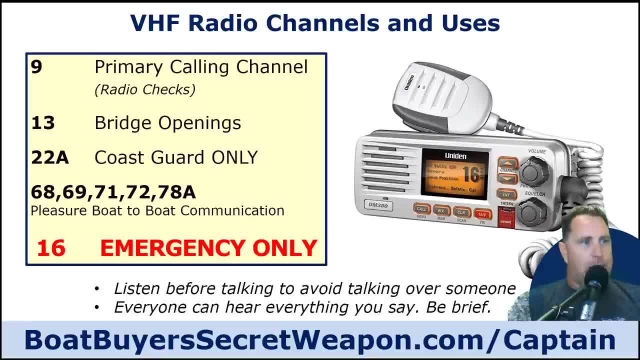 to know how. So number nine, channel nine, is the primary calling channel. That's where you say: hey, buddy, I want to talk to you. Go to channel whatever the pleasure boating communication channel If you're getting to a bridge, channel 13,, the Coast Guard's got 22A and channel 16. 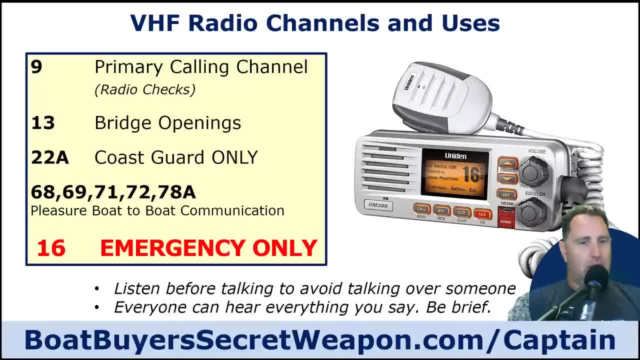 is the emergency only channel. That's not the channel. you tell your buddy where the fishing spot is or that you're going to your favorite cove. You call them on nine and say you know 27,. Sea Ray calling 16 Larson. 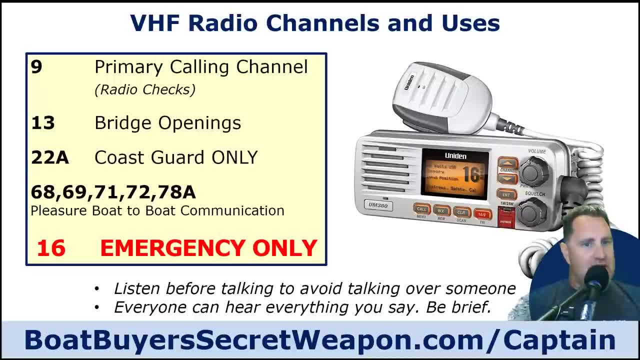 Go to channel 68.. You go to channel 68, and then you say, hey, we're going to Papa Doc's to grab some lunch. We're going to head out, We're going to this fishing spot. It's hot, That's where you. 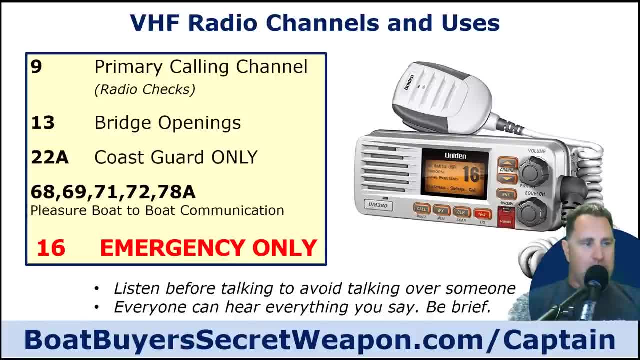 have those conversations, Always listen for a little bit before you start talking so you don't talk over somebody. Remember, everybody are on the same channels and us pleasure boaters have our own 68,, 69,, 71,, 72,, 78,. and be brief because everybody can hear everything that you say. It's 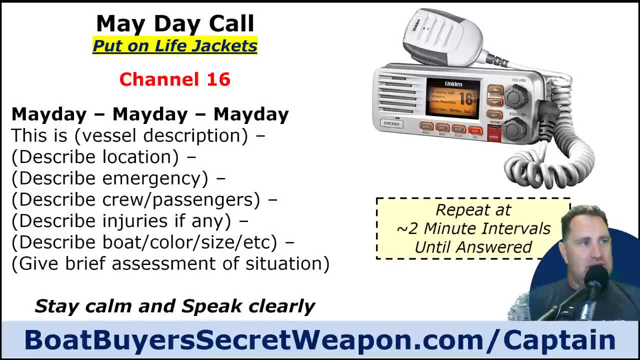 all on the same channel. We're polite. Channel 16 is for emergencies. Remember, if you do need to call a mayday, things are going down. Put on your life jackets first. Dial up, call 16, and make this. 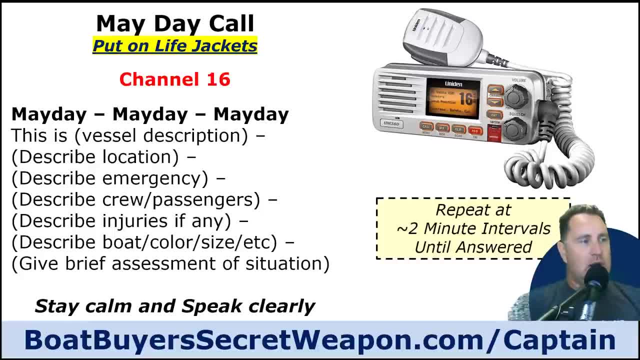 type of call: Mayday, mayday, mayday. This is 28 Sea Ray Latitude and longitude. if you know it are some sort of location description. Describe the emergency: We are taking on water and we're going down. Describe the crew and passengers. We have six people on board, three kids. 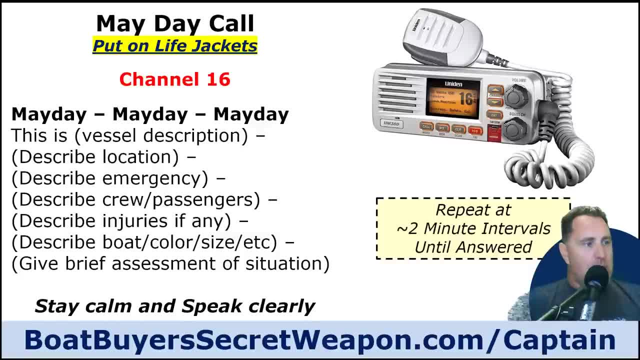 three adults. Describe any injuries: We have a broken arm or we have somebody that is having a seizure. Describe the boat color so they can find you. We are a red hull with white gunnels, size 28, with whatever defining markers you have on the boat, and then give a brief assessment of the 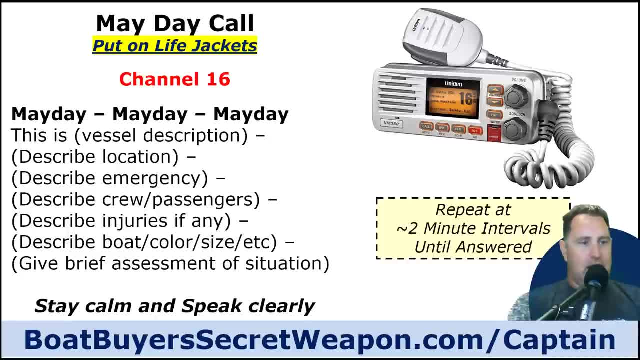 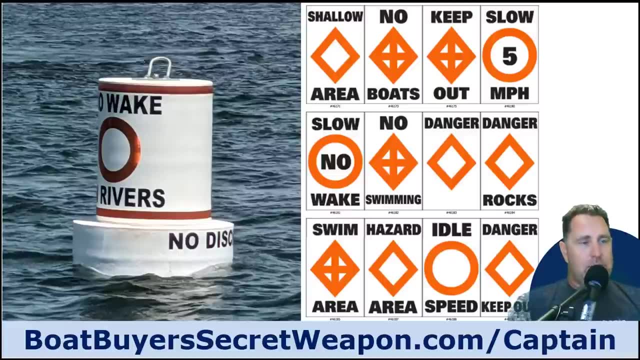 situation. Stay calm, Speak clearly. I know it's an emergency, but that will help you get better results. and then repeat that about every day, Two or so minutes until your call is answered. So now you know that Buoy markers. If you see something white with orange, it means there's a danger. If there's 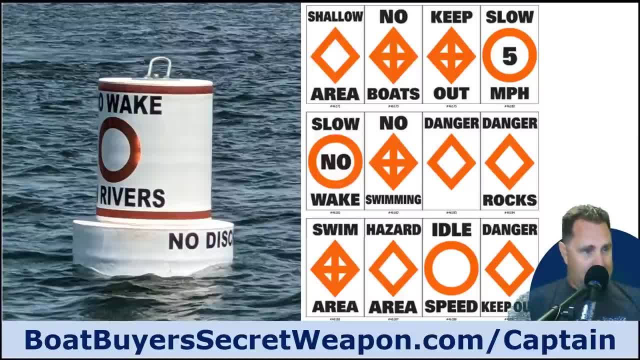 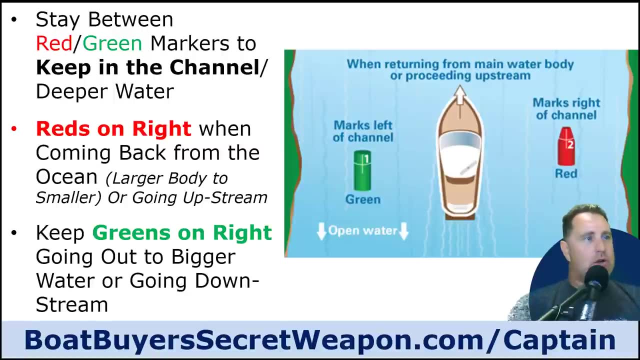 a circle, it means reduce your speed or go all the way down to no wake speed, idle speed. If it's a diamond, it means there's something in the water that you don't want to hit. So be aware, Know your signs. If it's a navigational aid, red and green markers are going to mark the channel. They're.